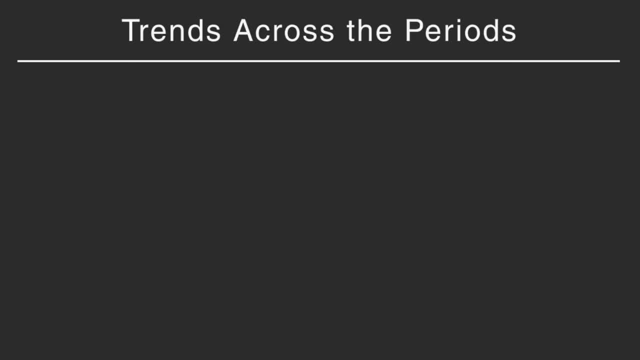 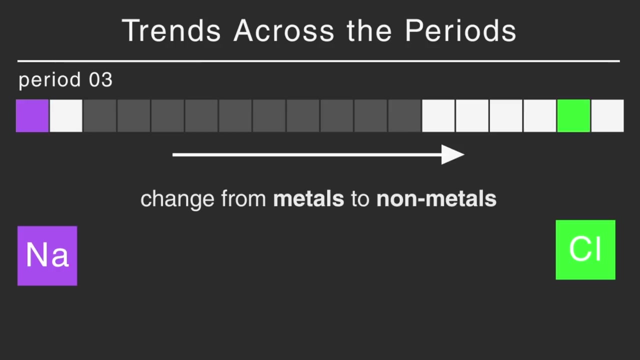 Let's take a look at the trends across the periods. Periodicity is the trend in properties across each period. Let's go from left to right across a period. What do you notice? First of all, elements change from metals to nonmetals. 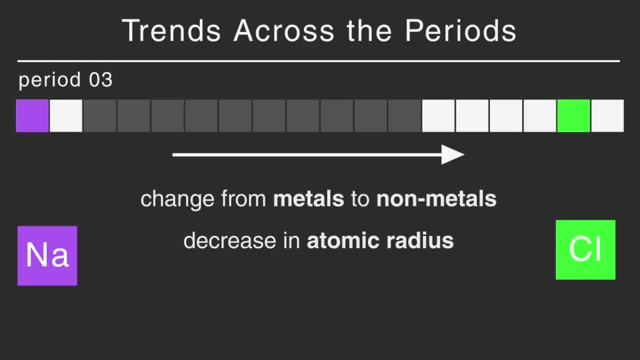 Also note that there is a decrease in atomic radius. This is because more protons are in. this is because more protons are in the nucleus, which pull the electrons closer in. There is also one energy waffle Here. you can see that the electrons have gone in and the children weren't formed. The elements and other protons are changing. 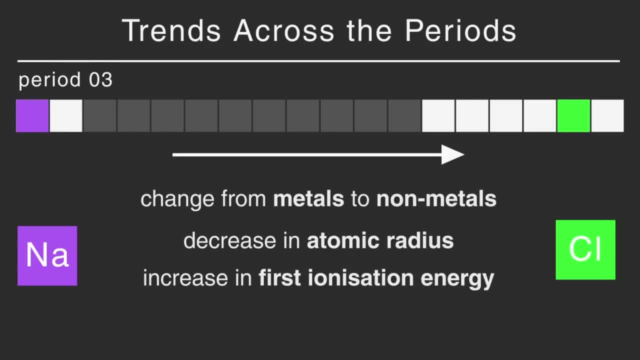 an increase in first ionisation energy, which is the energy needed to remove the outermost electron, and an increase in electronegativity, which means the attraction of a bonded atom for the pair of electrons in a covalent bond. Now let's look at the trends as we go down a group. 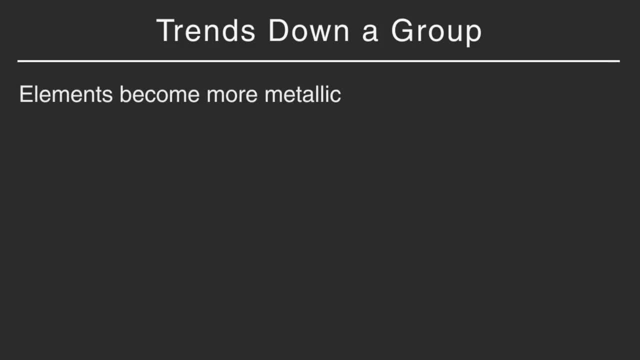 Notice that the elements become more metallic. This is clearly seen in group 14, where carbon in period 2 is a non-metal, but lead in period 6 is a metal. By the way, do you remember that metals are elements that react by losing electrons and non-metals are elements reacting by gaining? 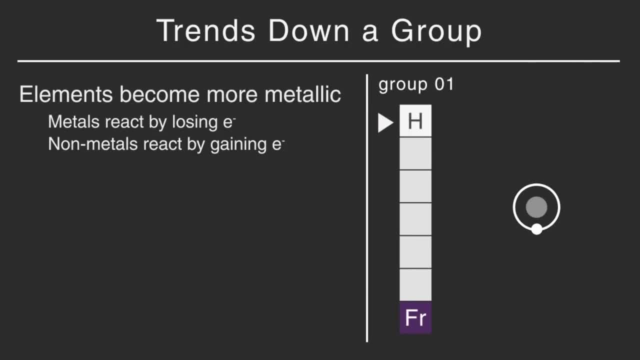 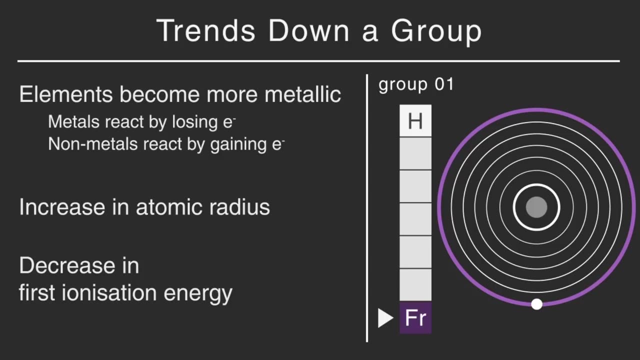 electrons Also going down the group, there is an increase in atomic radius. This means that an extra shell of electrons is added for each successive element. However, there is a decrease in first ionisation energy, which, as noted before, is the energy needed to remove the outermost electron. 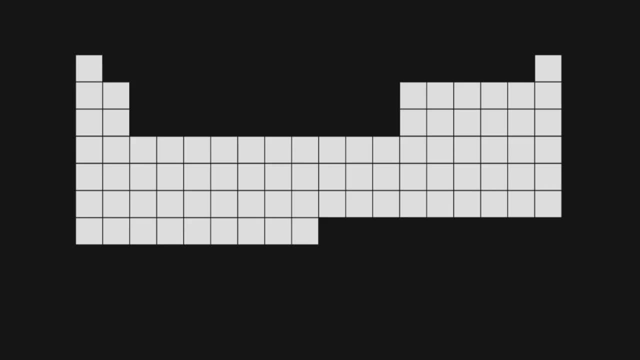 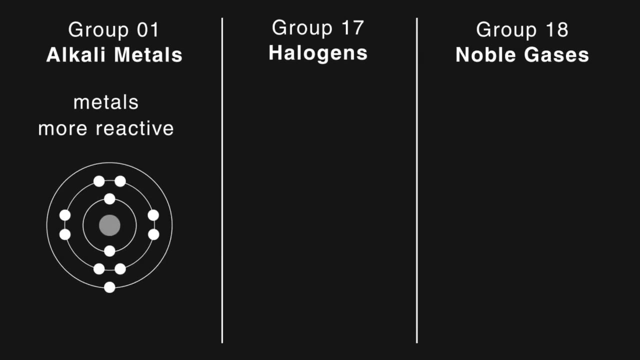 There are three groups of the periodic table that are usually studied: Group 1, the alkali metals, group 17 called the halogens and group 18 called the noble gases. As we go down group 1,, the metals become more reactive. This is because metals react by losing. 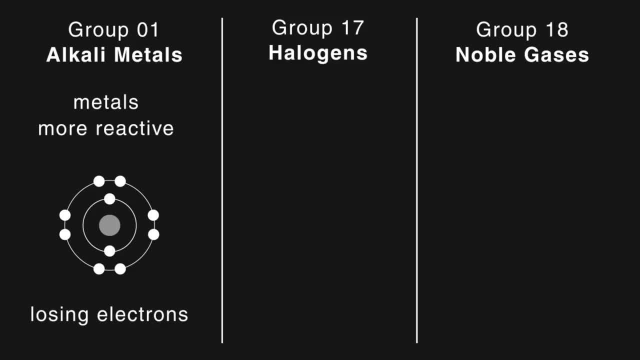 electrons and it is easier to lose the outer shell electron the further it is from the positive nucleus As we go down group 17,. the non-metals become less reactive because non-metals react by gaining electrons, and the fewer shells, the greater attraction for the incoming electron. 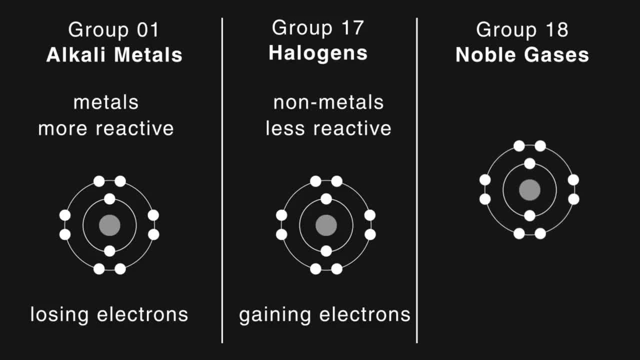 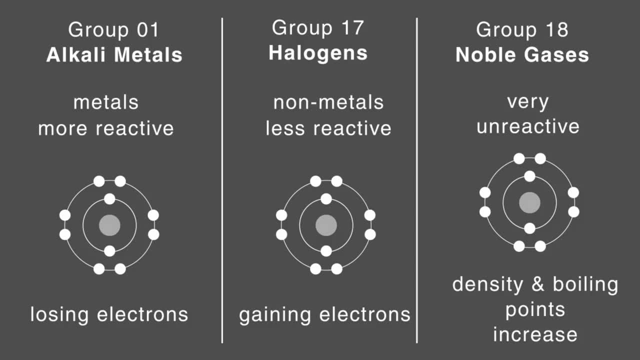 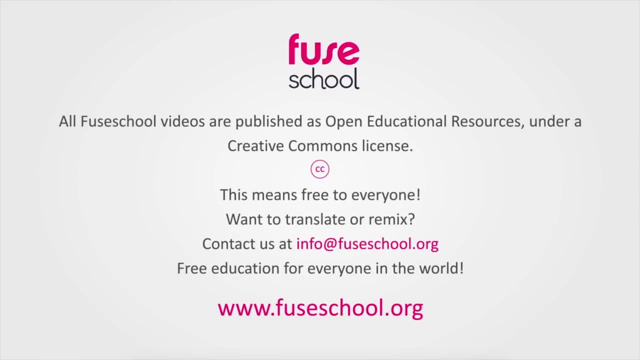 And in group 18,. elements have a full outer shell of electrons and so are very unreactive. Their densities and boiling points increase on going down the group. This means that Bangor is one of the most kept-on projects. For more information, visit http//wwwcanadacomuk.